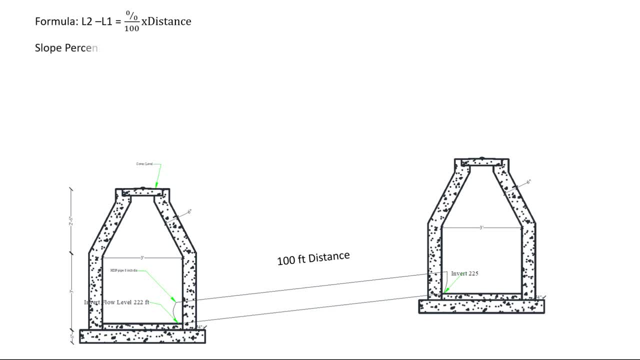 percentage into distance. we arrange this formula. First, to find slope, We are going to put values in l2, l1 and distance values below given values. The slope minus show the direction downward. we here draw arrow. Now we calculate slope to each 25 feet interval distance. 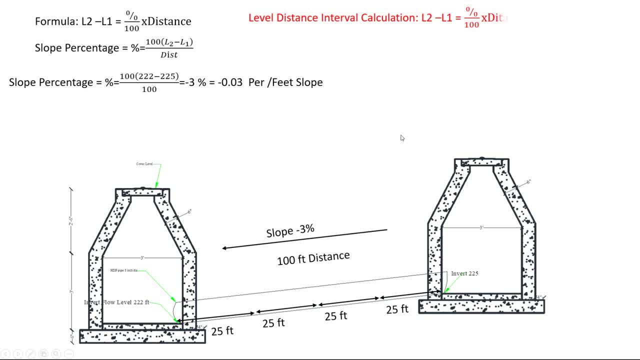 Now here, requirement: the formula arrangement for Casio calculator. we are going to advance technique: how to quickly calculate slope, interval distance on site When we working on site and how to solve this on site. The value of slope: already we calculated 3% divide by 100. we have here, per feet, slope minus. 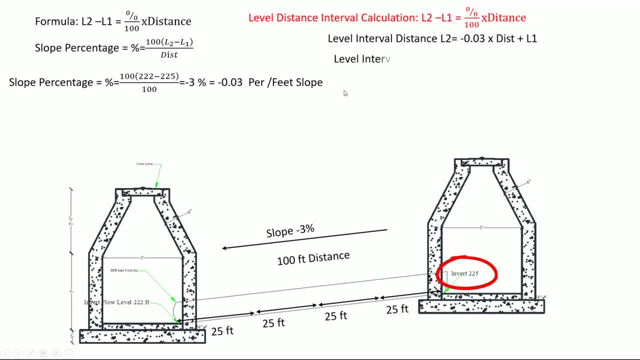 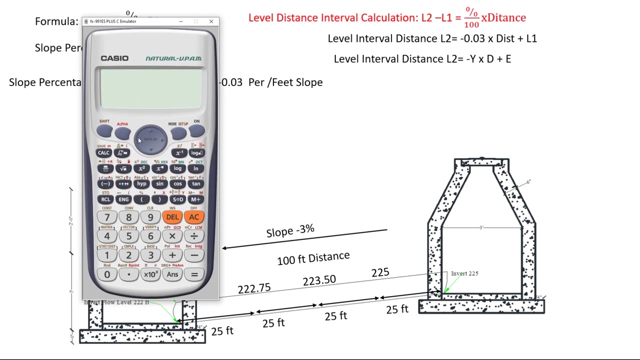 0.03 into distance plus l1 level. This formula for Casio calculator. We first showing levels interval here, Then how to prove it. To convert triangle into circle type in calculator: minus sign, press alpha and press y for slope, press alpha again. multiply d for distance. 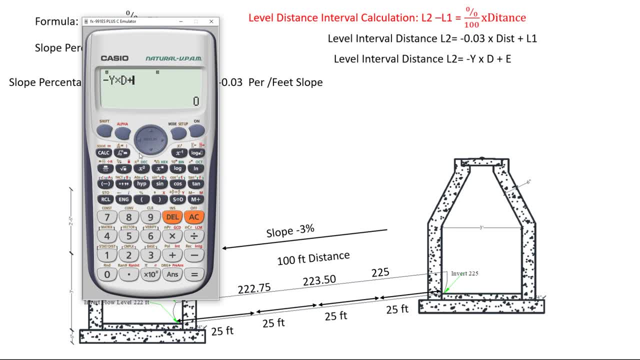 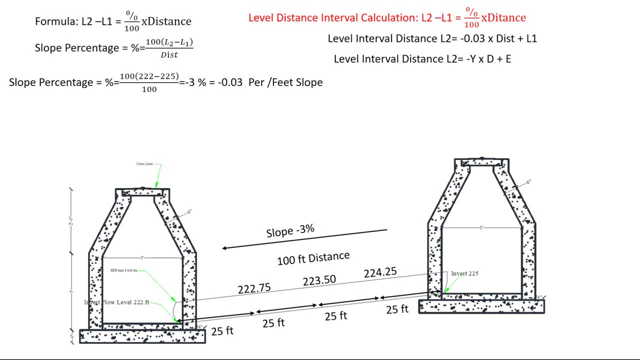 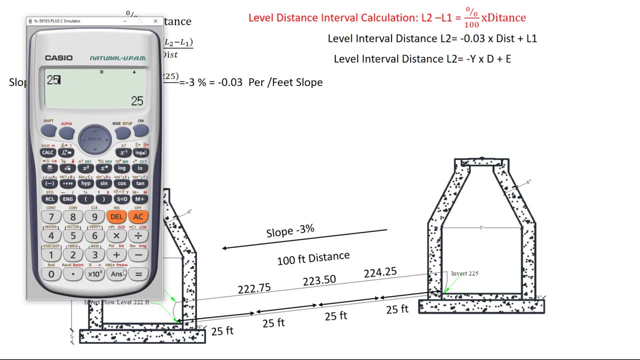 and plus E for level L1.. Now press on calculate button. Now they working automatically the formula Now: type 0.03 value for slope Distance interval. require level on 25 feet. Type value L1. press equal sign calculator. Now you only type distance interval value. the levels automatically calculated. 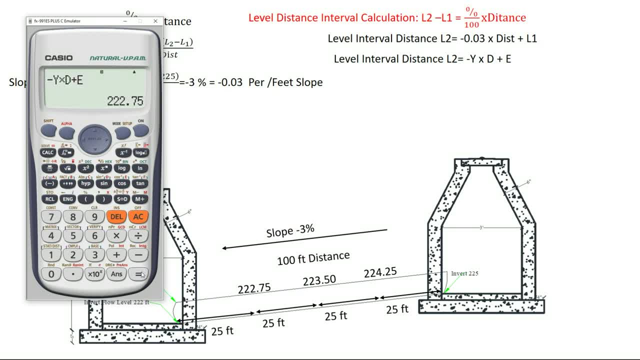 Type distance value: 75 feet press equal. the level is 222.75.. And the level is 222.75.. The last level on 100 distance is there Now, goodbye. thanks for watching.